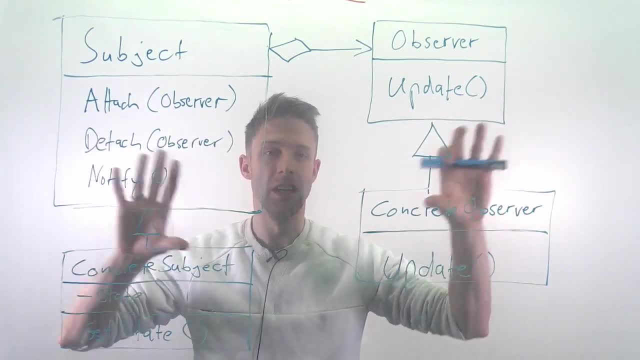 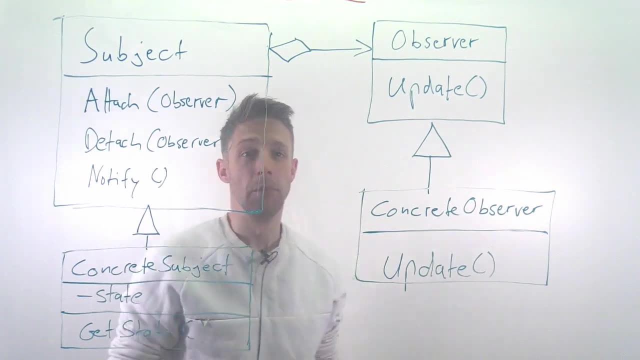 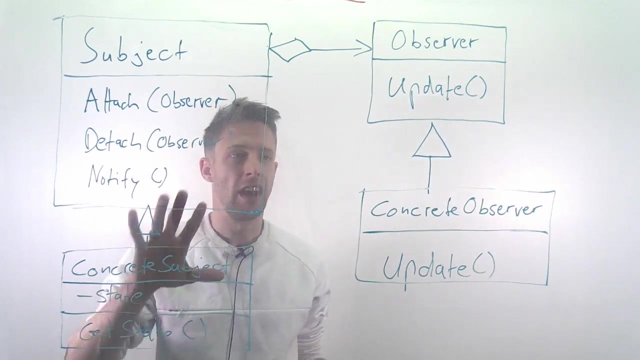 different part. So these are common things that so that you can evolve them separately and you can dynamically add, for example, multiple displays for the same data or multiple behaviors, multiple listeners for the same button. If you're not familiar with it or if you have forgotten it. 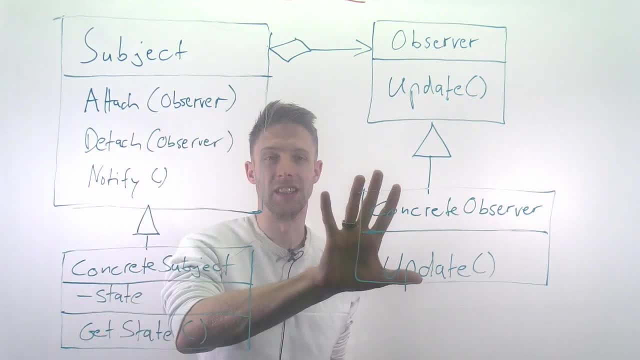 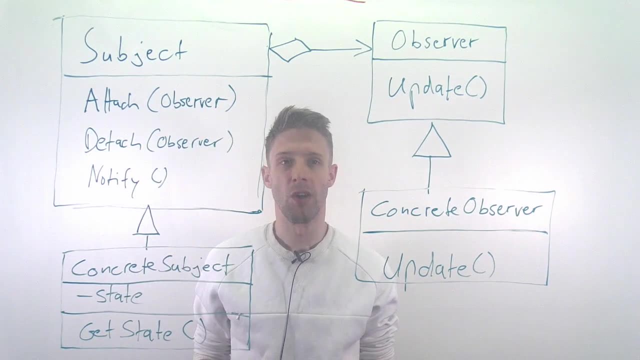 I would really recommend you to take another look at the class diagram syntax, because we'll use that a lot here. In particular, the object-oriented design patterns that we're going through all make heavy use of inheritance and things like polymorphism that, depending on if you call the concrete object the 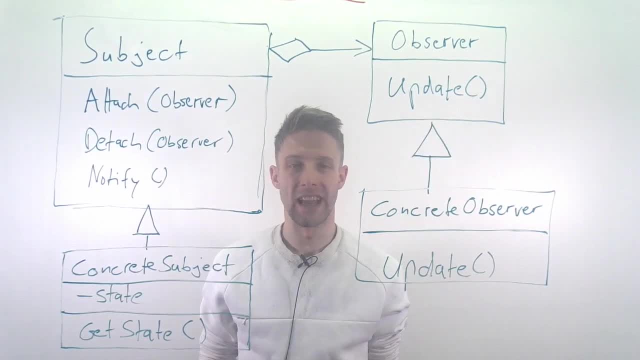 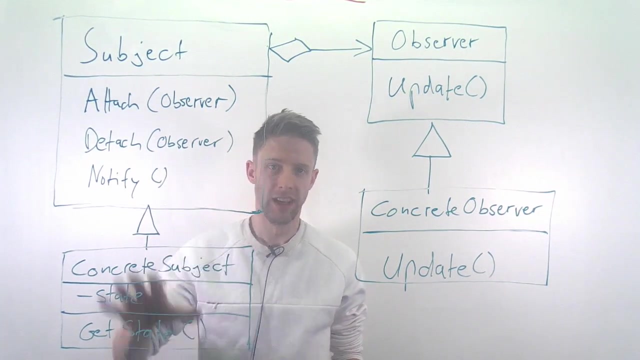 inherited subtype. then, depending on the language, you actually call the update function down here instead of the original one in the hierarchy In the parent class. So this is a behavioral pattern, the observer pattern. I'll just walk you through what this means. We have a subject that 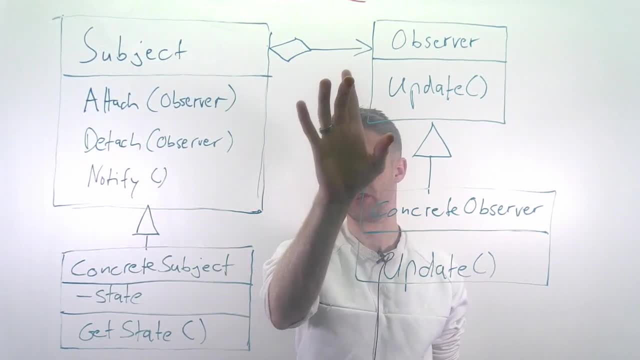 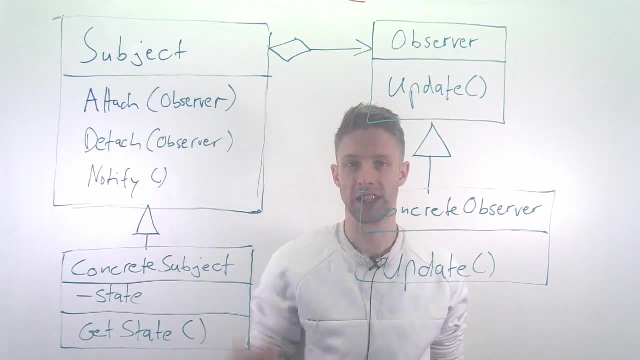 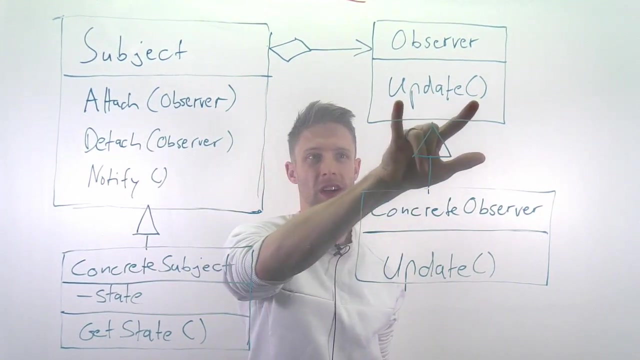 supports attaching and detaching observers, So you can, at runtime, call this method and say: I am an observer, I would like to attach myself to this subject, And then the observer itself has an update method. So this is how you tell the observer: something has changed. 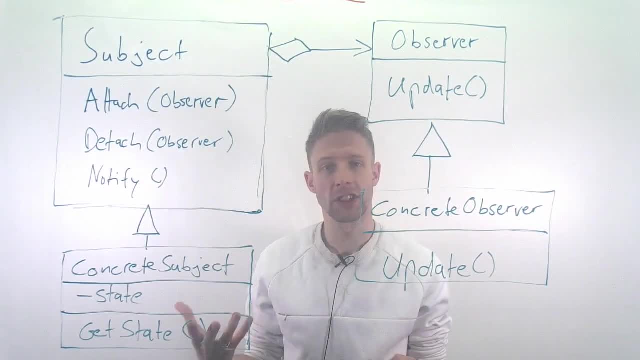 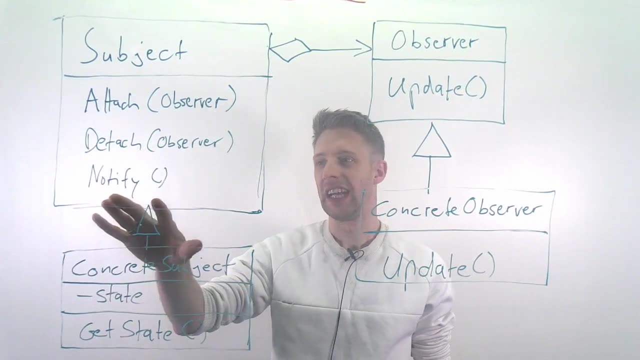 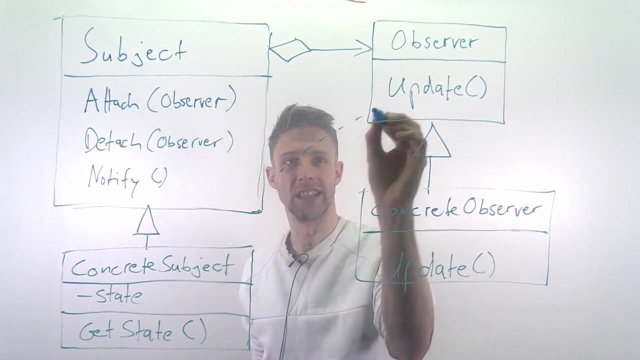 Now imagine the subject changes, for example, the data changes, you do something, the database. what happens then is that you call the notify method of the subject and the notify method of the subject goes through a list of all the observers and for each of these observers that basically calls the. 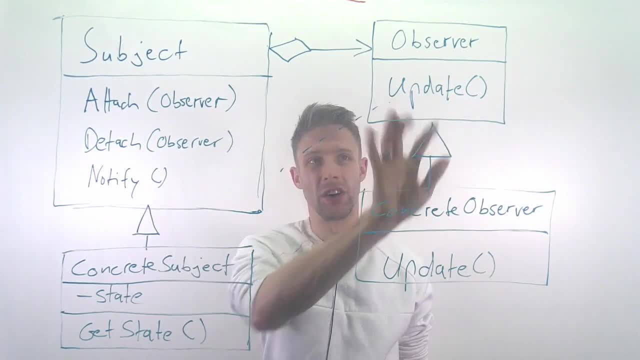 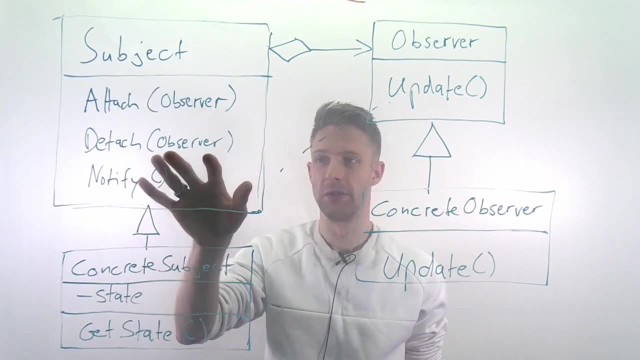 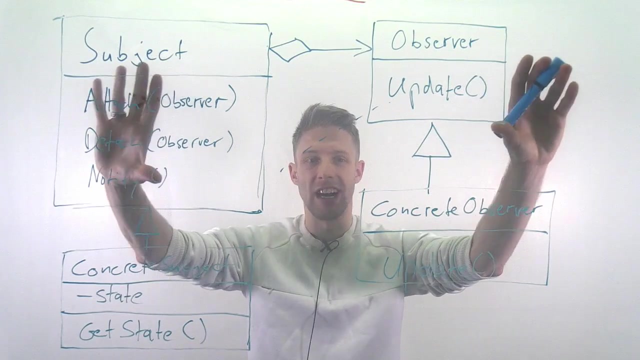 update method. So by calling notify, all of these update methods are called, and if you call detach again, the the subject simply removes the object observer from the list of existing observers. now that's sort of the higher level here. then you have the concrete observer and the concrete subject and 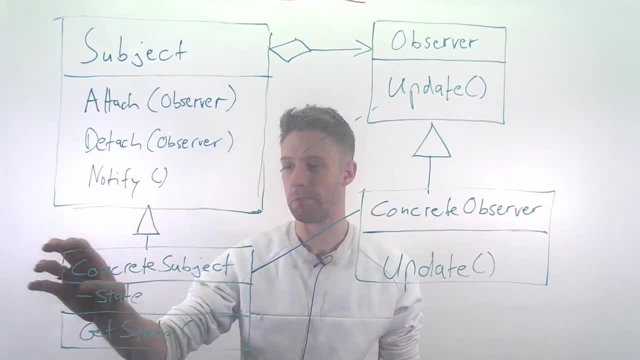 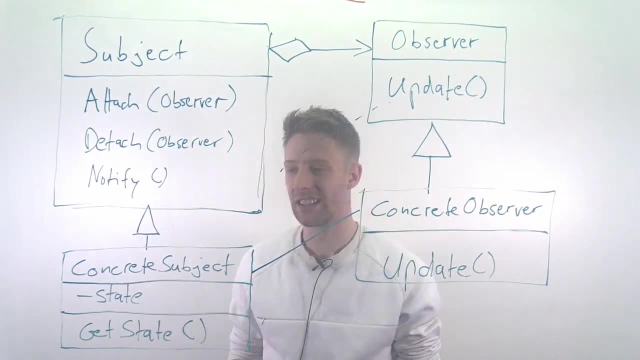 they actually need to know each other. so, for example, if you implement a button, then you have a button listener that knows exactly what kind of state the, the concrete class, has. if you implement some kind of data structure, then this information is here: how does the data structure look like? and the observer? 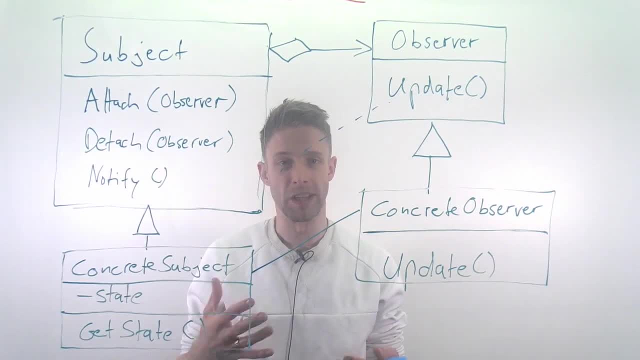 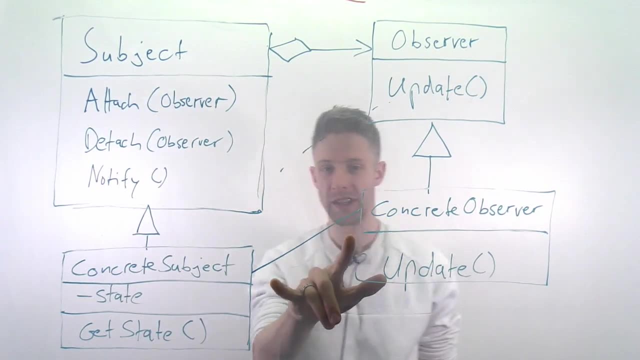 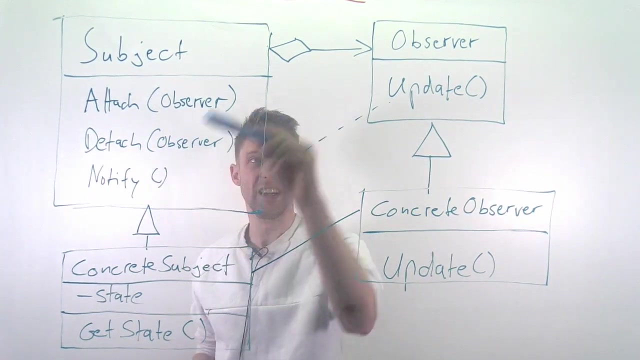 needs to know that, because if you want to- for example, let's say, you display a bar chart or a pie chart of that data- for that you need to know how the data looks like. so that's why you have this line in between here. the concrete classes know each other. so what happens if I call notify the update method here? 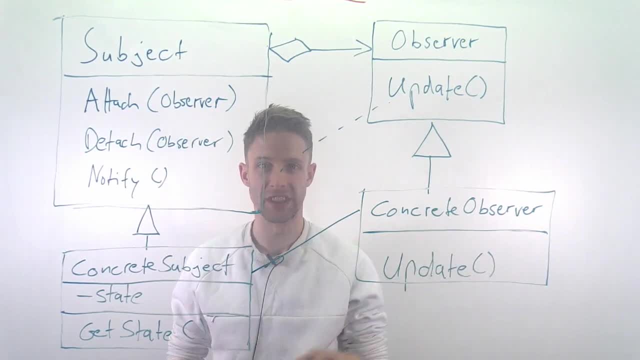 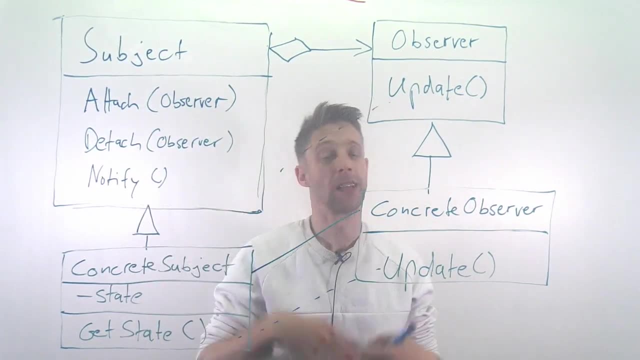 is called, and the concrete implementation of the observer then calls the concrete get state function. so basically, we tell the observer something has changed and the concrete one says: okay, I know what kind of subject I'm dealing with. I'll call the get state method and I get back the. 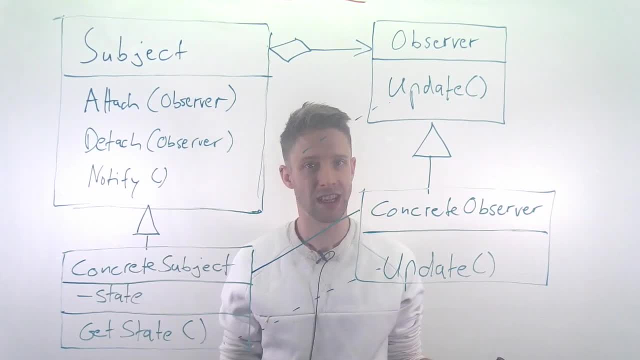 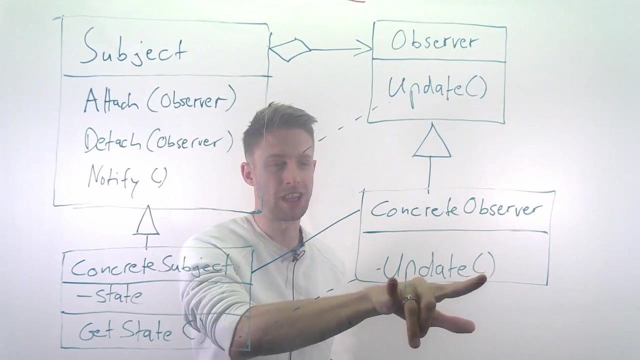 current state. so imagine now this is, for example, election data. our concrete class is some kind of implementation of this data structure: states, parties, votes, and we have an observer that displaced this as a bar chart, as you often have. once we call the notify the update, one here is called of our bar chart. the bar chart knows. 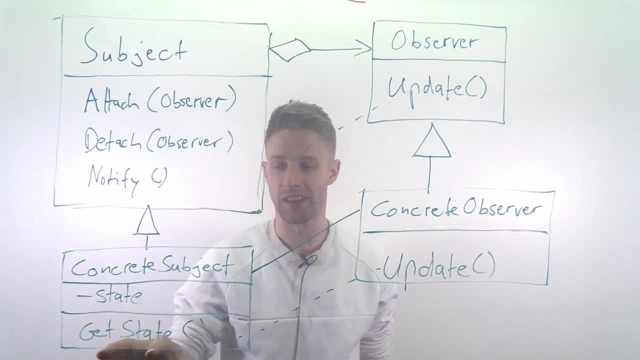 exactly how the data looks like. so it calls to get state method and they get. state method returns the state, which is the concrete data structure with the polling information, and then the observer updates the display. as I said, this is common, for example, for button listeners, so for any kind of listeners. 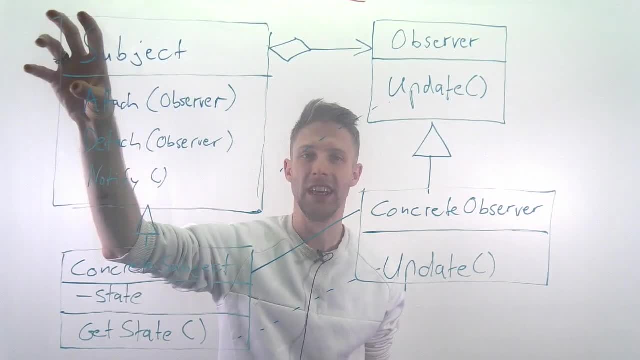 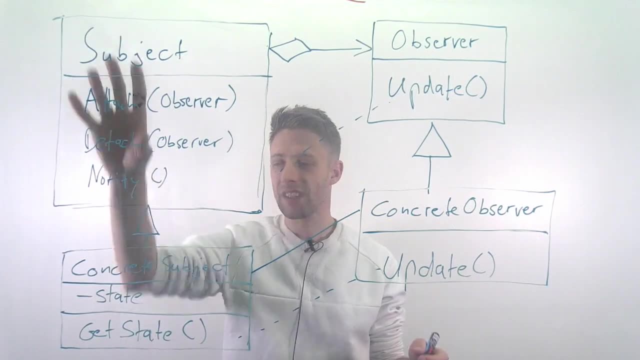 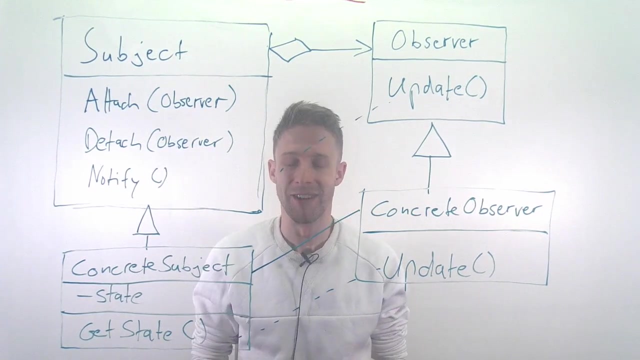 actually event listeners and programs. so, for example, here you would have a generic class button and you would have a generic class listener, and down here you would have a concrete implementation of the button and a concrete implementation of the button listener- listener, which is, for example, the case. 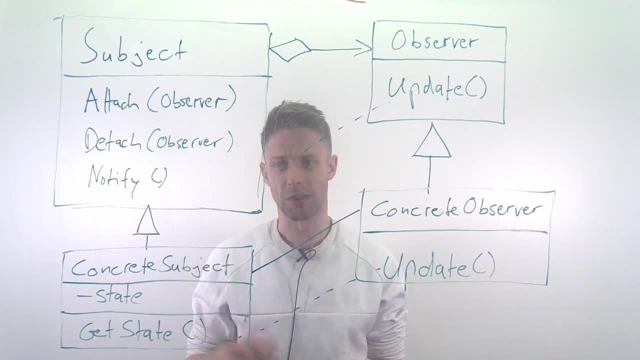 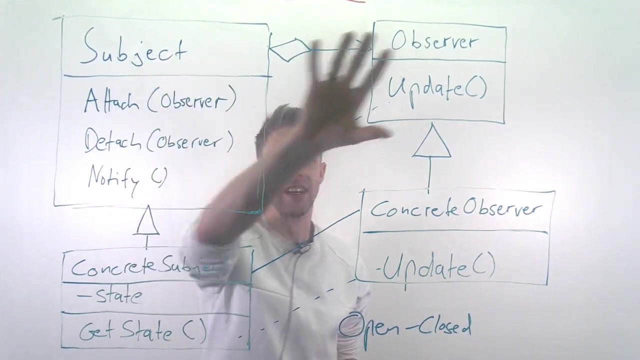 in Java, where you can do these kind of things. so that's one common implementation of the observer pattern in practice that you might come across. in terms of the solid principles, what we see here is, on the one hand, the, the open, closed principle, so these two parent classes are not made to be modified. 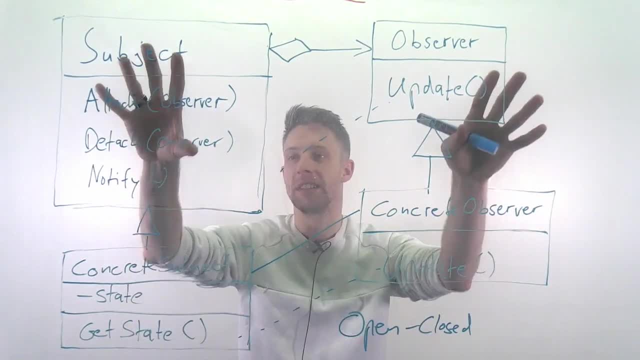 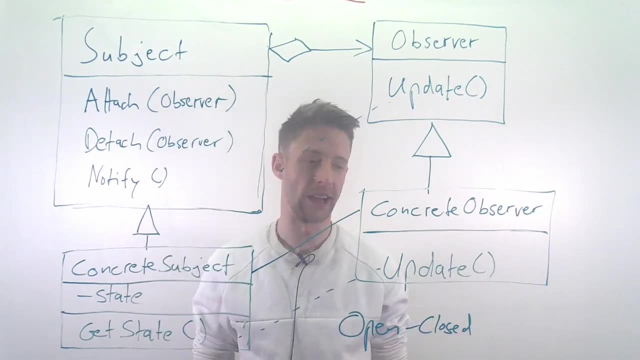 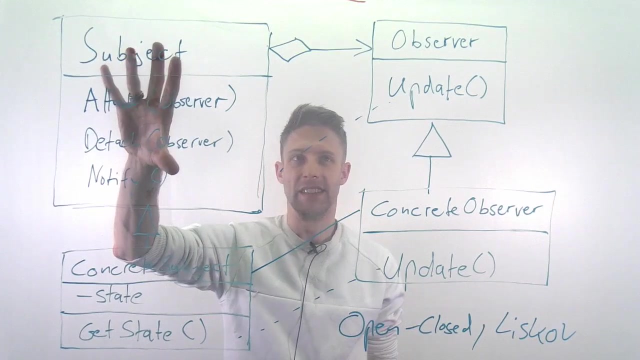 they're kind of fixed, so they're closed for modification but they're open for extension. so the idea is that you add things on top of them. that's the open- closed principle in practice, basically. and the other thing we have here is Liskov substitution, so the abstract type, subject and observer, we can at any time.